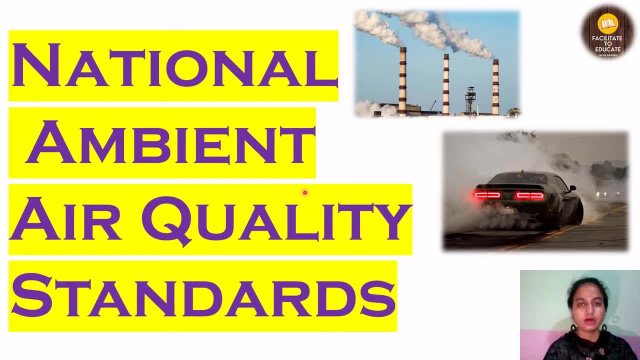 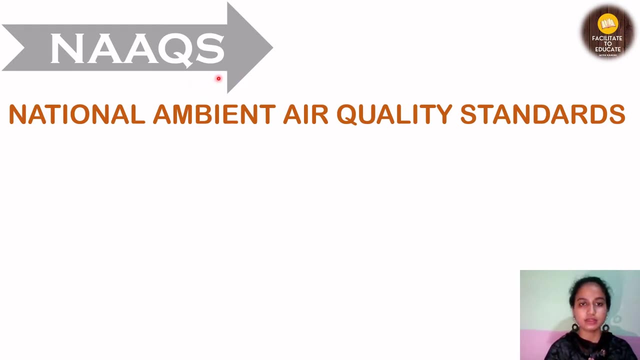 that you are going to give or will be giving In NET examination also. paper 1 and paper 2 are important for both. So first of all let's see some general information. NAAQ is its short form. Please remember that you can ask in this form also, So don't get confused. 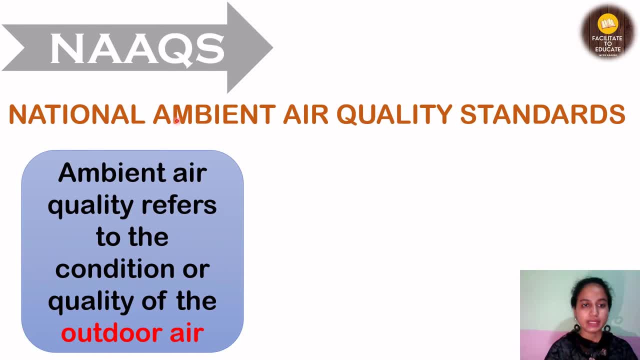 about what it means. So, first of all, National Ambient Air Quality Standards. What is Ambient Air Quality? Ambient Air Quality means outdoor air, that is, the condition or quality of the air outside our house or our building. So we will call it Ambient Air Quality. 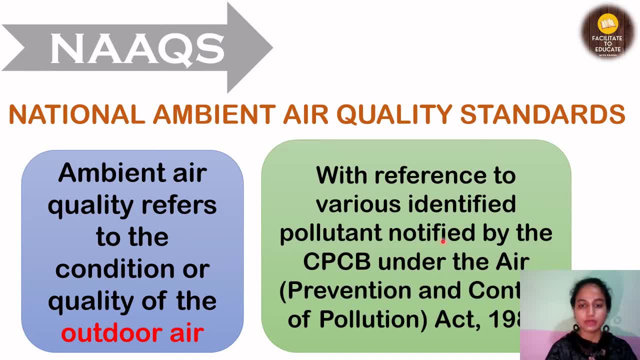 So what is Ambient Air Quality? Ambient Air Quality is the condition or quality of the air outside the building or, in general, any building you have. Our smile is 되어. naai kahe di comli. So Ambient air Quality is a condition or quality of the air outside. 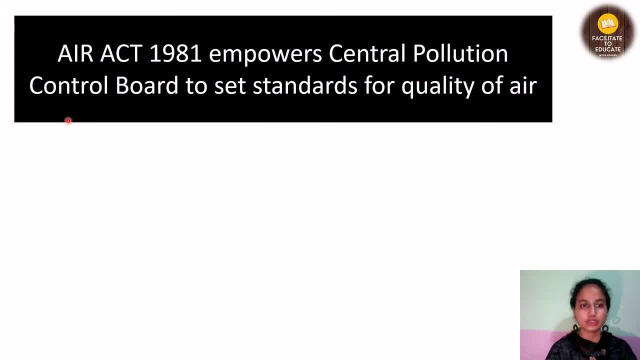 our house. they areеб kudke hai Fabrikat hai Sabisey. So Ambient Air Quality is a condition of the air outside our house. So we can explain it: air quality standards. All these standards have been given since 2009, ie they have been given many times before that. 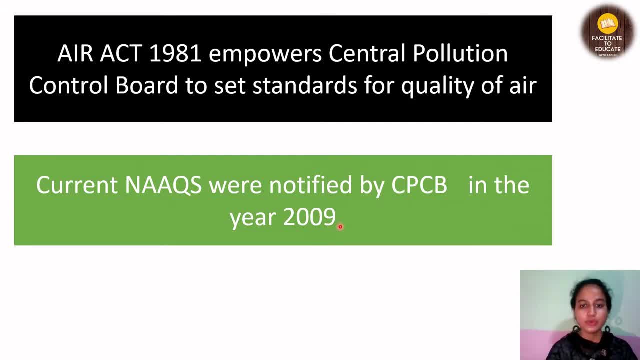 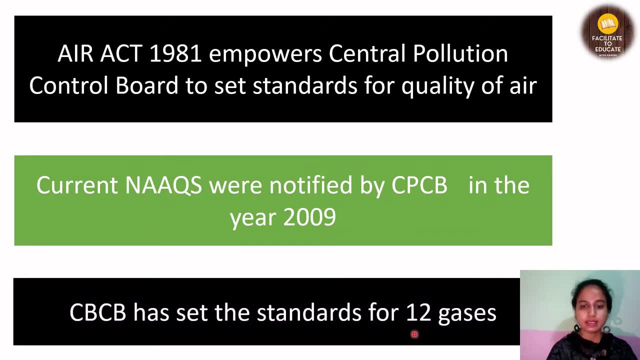 but the latest one was given in 2009, which we will talk about in this video, And these are for 12 gases. 12 air pollutants standards have been given. These are the major gases which were also discussed in the Air Act 1981.. 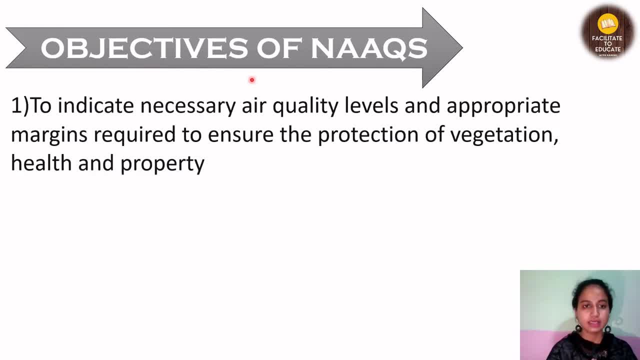 Now let's see the objectives of the Act. First thing is that we set some appropriate margins, ie some thresholds for air quality, so that our vegetation, health and property are protected. Second thing is that uniformity should be given in the national level of air assessment. 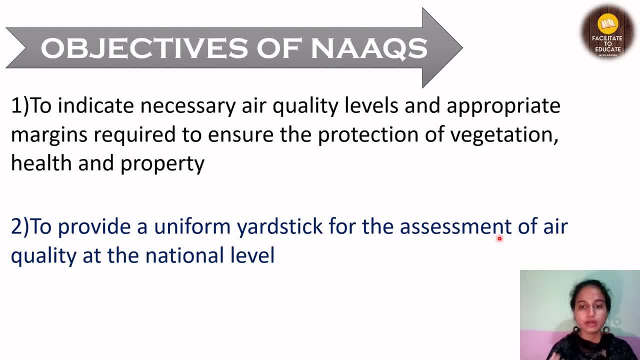 ie if we are doing the air quality and air quality assessment and we are assessing it at the national level, because states can give different standards, but if it is done at the national level, then it is more fruitful and helpful for us to know that. how is the air quality of every place? 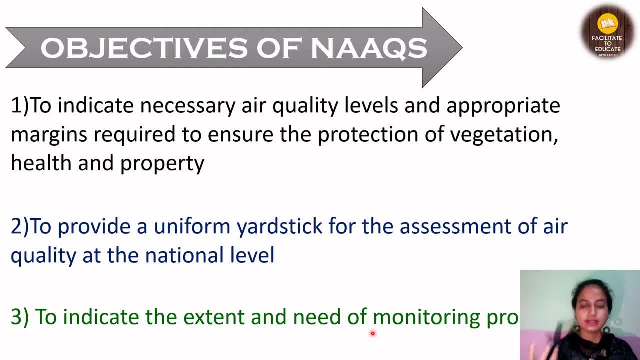 And the extent and need of the monitoring that we are doing, how to do it, to what extent should it be done, and the need for it. also focuses on that and tells us about it. So these were the three major objectives. There are some minor objectives as well. 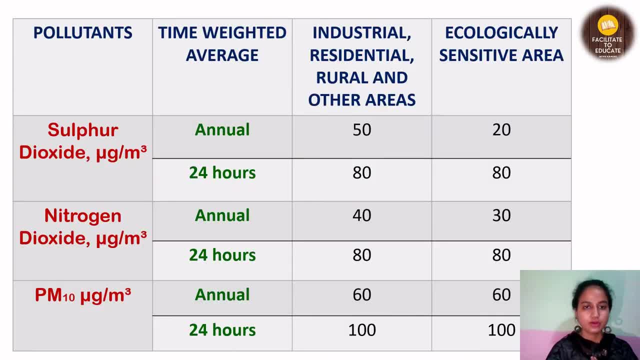 But these three are the major objectives. So now let's see which gases we are talking about. What are the names of the 12 gases we were talking about? Second thing is that: what are the standards given for each area? So there are two types of areas. 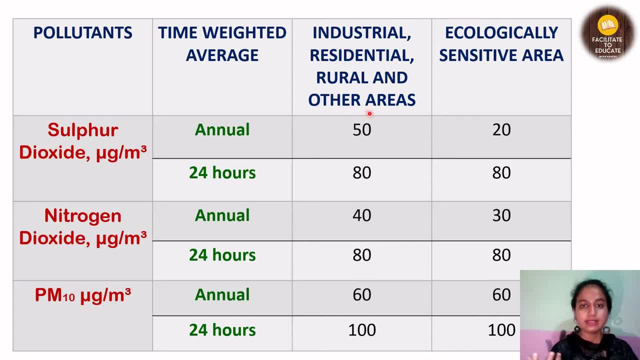 First is industrial, residential, rural and other areas. These areas have been given the first standard. Second is ecologically sensitive areas. These are the sensitive areas that CB has issued a list of which regions will come in: ecologically sensitive areas And industrial, residential, rural areas. 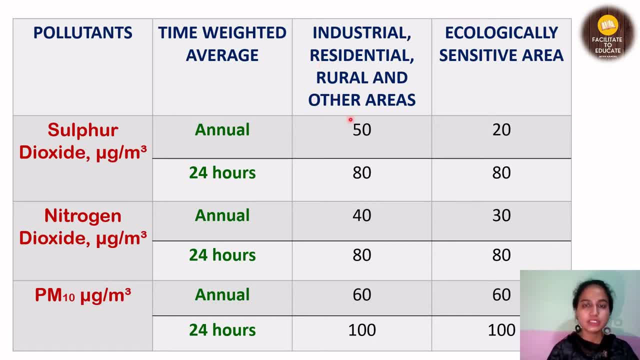 the areas in which we live, the areas in which there are industries, the villages in which we live. all these areas have been considered as one area. Second thing is the time-weight average, that is, for how long we are taking the average of that gas, that pollutant. 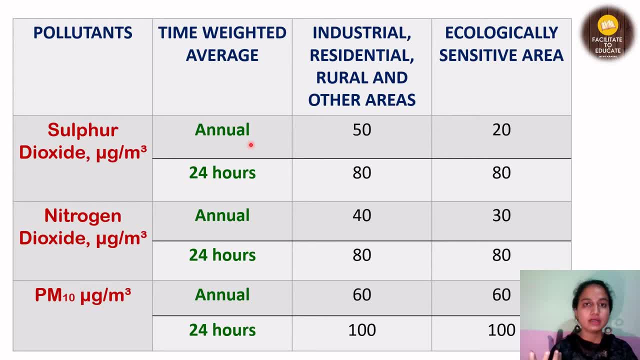 So there are some gases for which we measure them annually. That is how much of their standard should be in the atmosphere throughout the year. Basically, these annual gases should be measured at least 104 days a year. The second thing is that they should be measured twice a week. 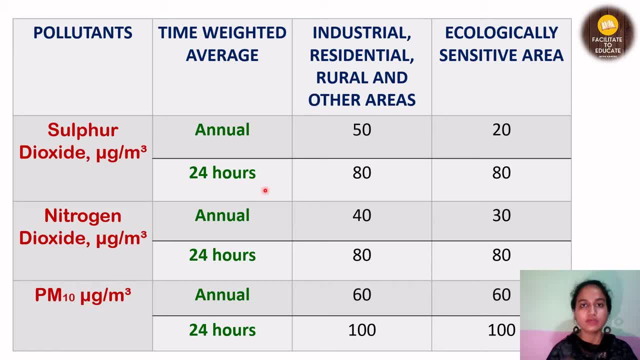 This is one of the rules. The second thing is that 24 hours or 8 hours or 1 hour- Whatever gases are measured For. now you are seeing that there are almost three gases for 24 hours. You will see further in the second list. which gases are measured for 8 hours or 1 hour. So all those gases should be measured at least 98% of the year, That is 98% of the year. The set standard should be shown in that. Only then we will consider it correct. 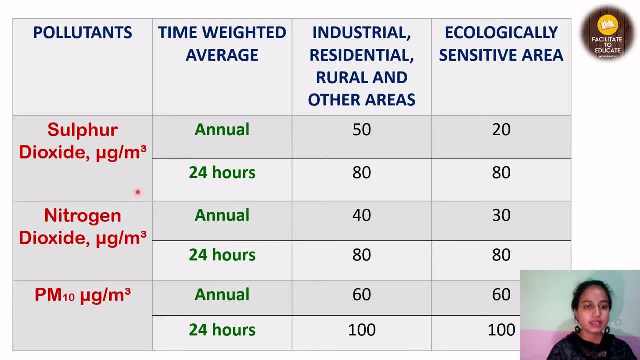 The first gas is sulphur dioxide. Keep watching its units. For now all the units are the same, But we will see further that for some gases the units change or become different. So for sulphur dioxide in the area number 1, there is a set standard of 50.. 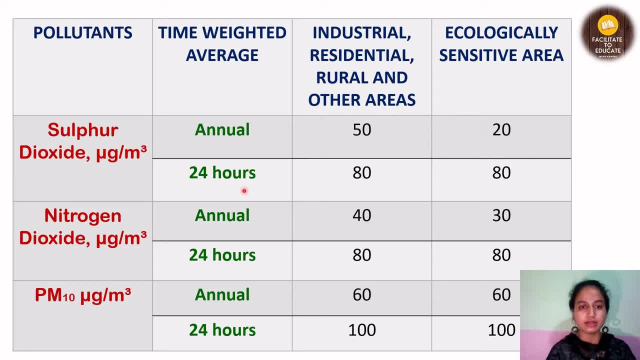 And in the ecologically sensitive area there is a set standard of 20.. For 24 hours, both are the same: 80 and 80.. For nitrogen dioxide, for annual 40 and 30. And for 24 hours, 80.. 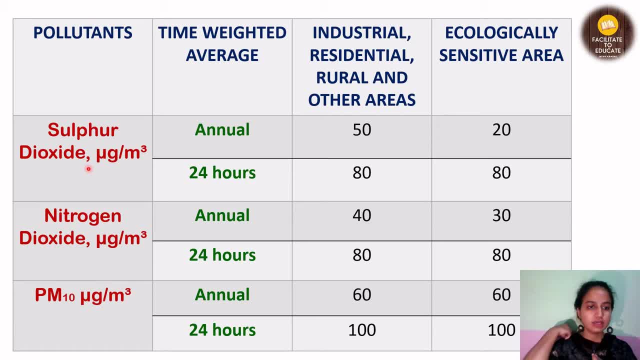 Same as sulphur dioxide. Same as sulphur dioxide. The second one is PM10.. That is particulate matter, 10. And its annual standard is 60 and 60.. For both areas And for 24 hours, 100 and 100.. 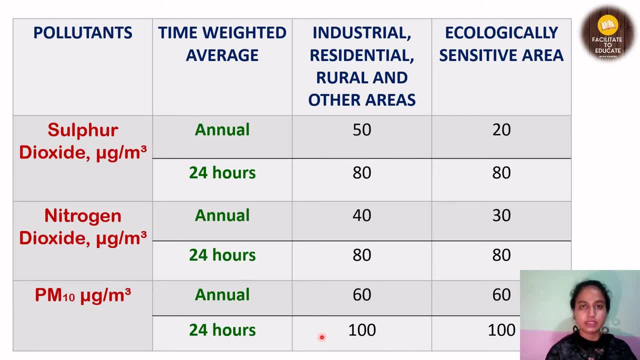 You will have to remember all these standards, measurements and numbers, Because any gas can be asked. Any gas can be asked. Major gases: There are 6 major gases: Sulphur dioxide, nitrogen dioxide, PM10, PM2.5, carbon monoxide, lead. 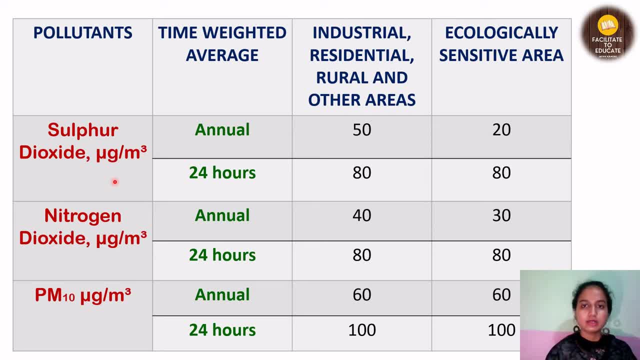 All these gases are repeated questions in competitive exams. Other gases are there. The standard is also set for them, But they are not that important. Most of them are not asked in exams. If you remember, then remember all of them. It is very easy to remember the numbers. 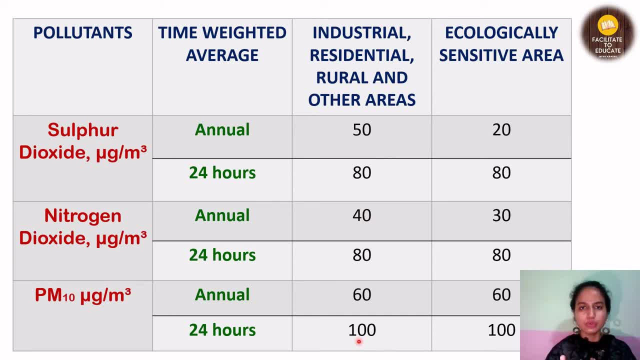 It is not hard. There are many gases for which the same values are given for both areas. Next is PM2.5. Which is 40 and 40 for the annual measurement And, for 24 hours, 60 and 60 for both areas. 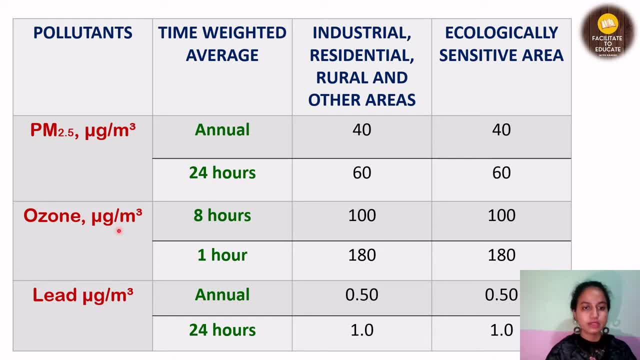 Talking about ozone. the units are the same for all three, But one measurement of ozone is taken for 8 hours And the other is for 1 hour. So in this there is no annual measurement, There is no 24-hour measurement. 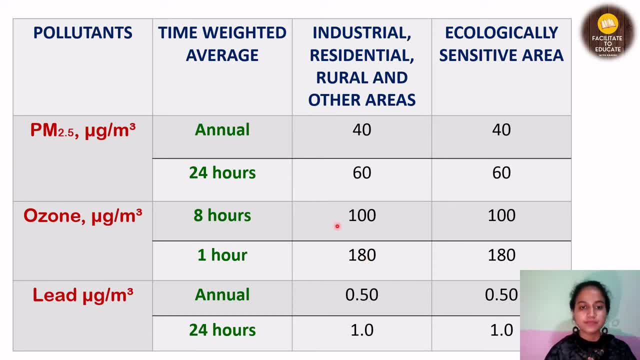 There is no 1-day measurement In this, there is only for 8 hours and 1 hour. So in this the first area is 100 set for both areas, Which is an 8-hour measurement And which is 1 hour. 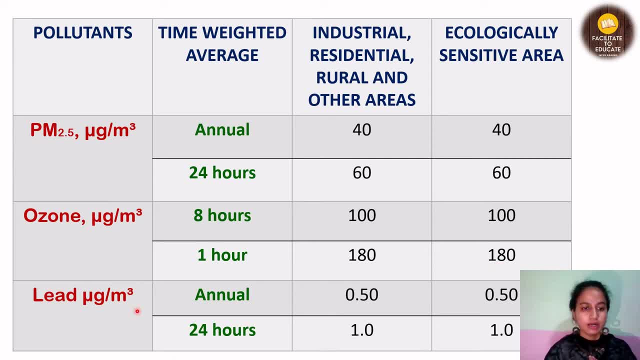 For that there is 180 set. Then there is lead, For which 0.5 means very less standard is set for the annual, Because it is a very toxic gas And if it enters the atmosphere then it is very difficult to degrade it. 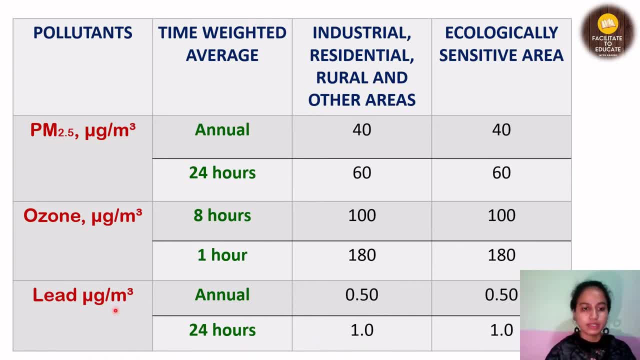 Then for 24 hours, it is 1. Microgram per meter cube For all these. as far as we have seen, the units are the same. Next is carbon monoxide. Its unit has changed: Milligram per meter cube. 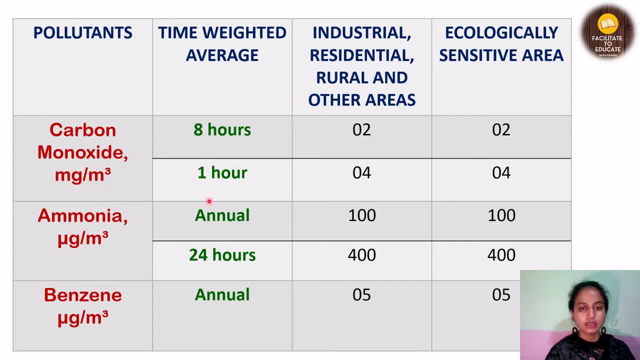 Be sure to pay attention to this. Second thing: this is also measured for 8 hours and 1 hour. Its set standard is also 2 and 4.. That is, it is very less. Then there is ammonia. Again, the same unit is set for the annual and 24 hours. 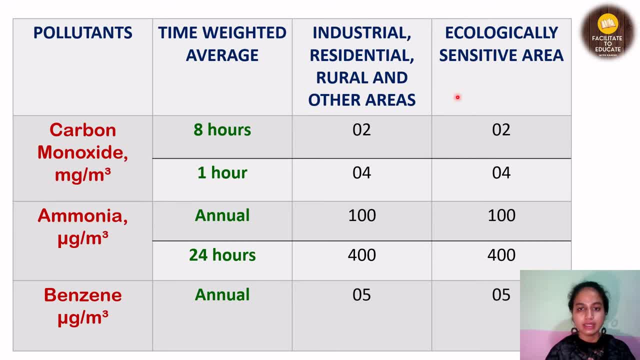 Which is 100 and 400 set for both areas. For benzene, its measurement is only for the annual. There is no measurement for 24 hours, 8 hours or 1 hour. For the annual measurement, its value is 5 and 5.. 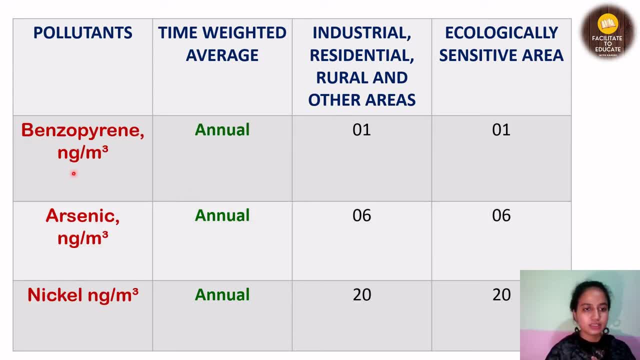 For both areas. Other than that, some gases like benzopyrene, arsenic and nickel- The units have also changed for them. You can see that all three have the same unit And they are measured annually. For benzopyrene, there is one standard set. 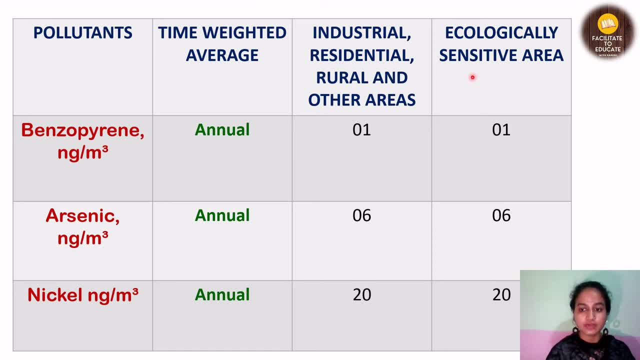 That is for both industrial areas and ecologically sensitive areas. Then for arsenic it is 6 and 6. And for nickel it is 20 and 20. So I will repeat it again, What you have to keep in mind. 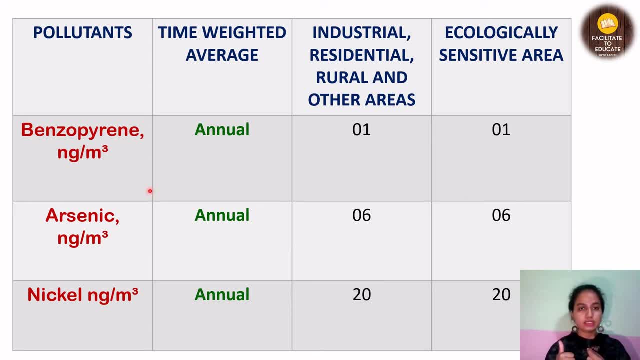 First, what are the names of 12 gases? What are the names of 12 pollutants? Second thing is for how long they are being measured. What gases are being measured? for 24 hours Or for the whole year? For 8 hours? 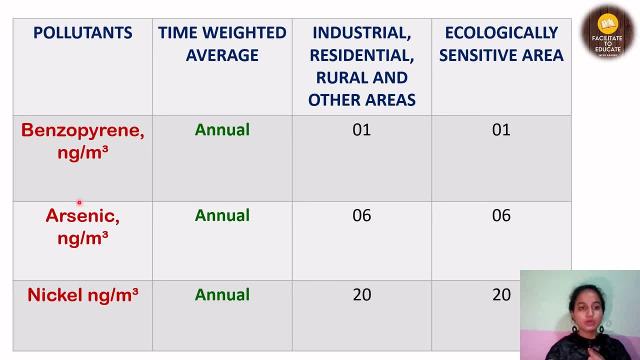 For 1 hour. You have to keep this in mind. In which unit are they being measured And what are the two different areas for which they are being measured? These are the general questions. You have to remember the other values. Any value can be asked. 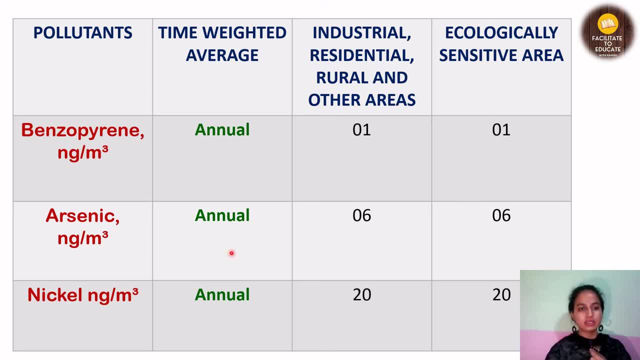 Major. I have told you that there are 6 gases. Otherwise, arsenic, nickel, benzopyrene can also be asked. There is no such hard and fast that only 6 gases will be asked. So, if possible, remember all. 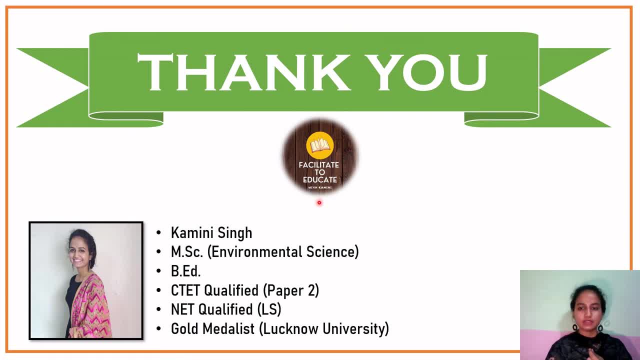 I hope you have understood the whole video well About National Ambient Air Quality Standards. If you have any doubts, you can ask in the comment section And you can also follow me on Instagram. The name of the page is Facilitate to Educate.